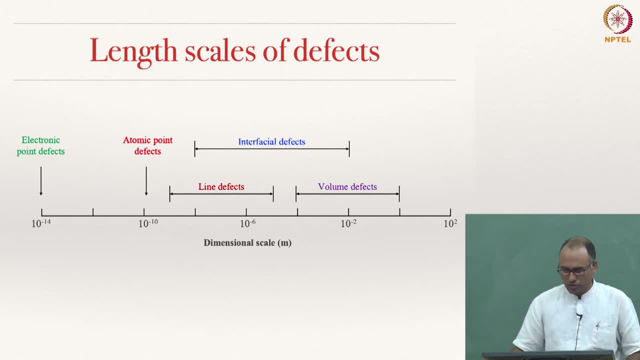 working at the order of angstroms, right, And when you are talking about line defects, you are actually talking at the scale of microns, 10 power minus 6 meters, couple of tens of nanometers or hundredths of nanometers to microns, 10th of micrometers And interfacial defects. 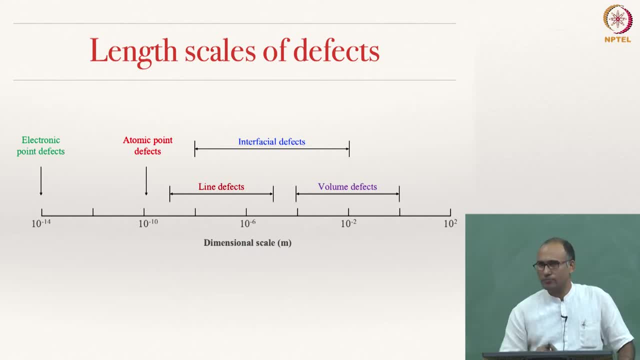 they are actually having much higher length scale than the solid, and it is completely accomplished. and your line defects? they can actually start from at the micron scale to millimeter scale. And then you have volume defects. usually these volume defects can be observed with 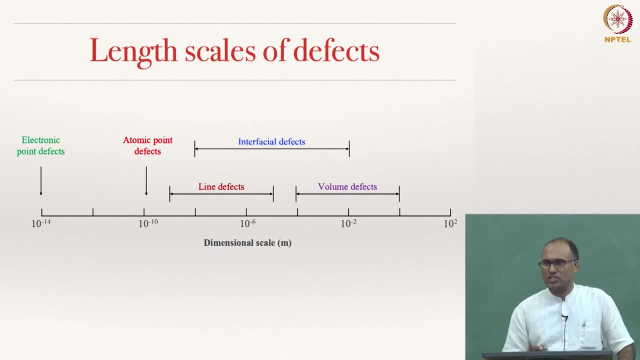 naked eye, Whereas line defects and interfacial defects are usually not observable with naked eye. you need to look under a microscope to actually identify these line defects and interfacial defects. So if you want to look at atomic point defects, you need to have a much more powerful microscope. 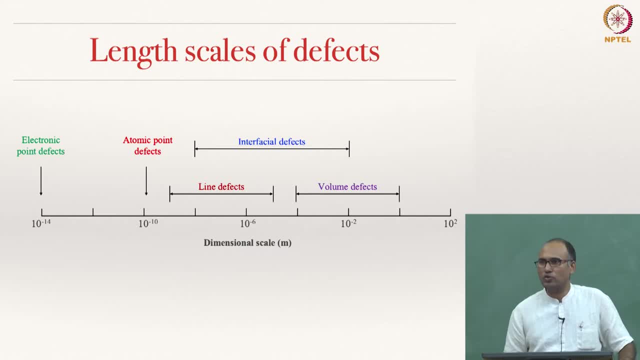 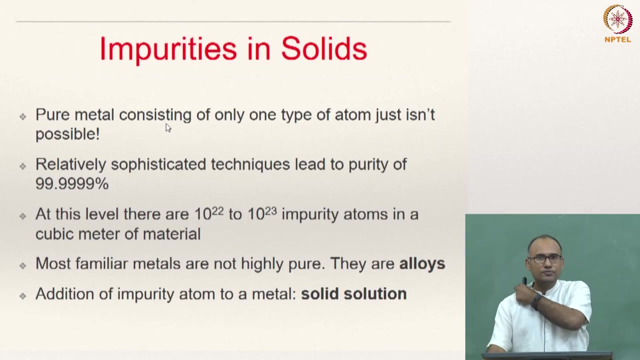 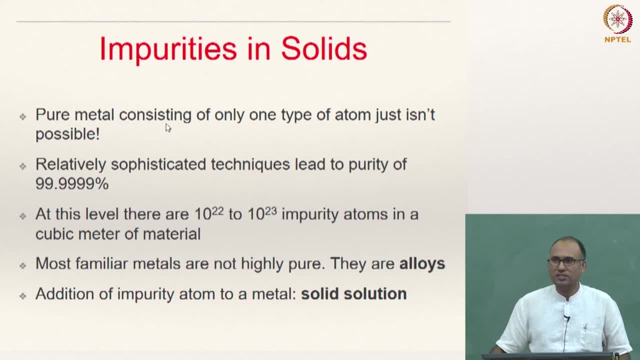 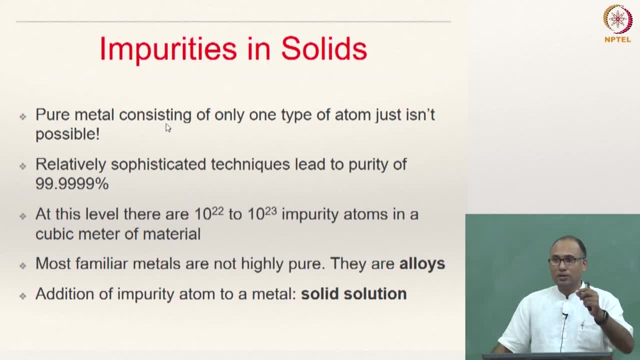 of vacancies. I am only. I am actually talking about existence of some other material. Just iron is simply not possible. just copper is simply not possible. If you have extremely sophisticated methods to extract these materials, you can literally reach up to 99.9999% of purity. even when you buy gold, they will give you the purification. 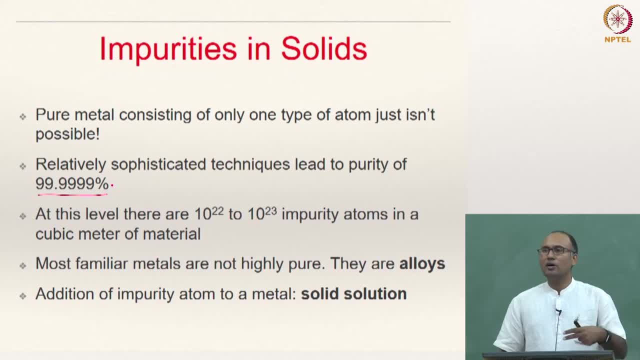 number. So that means if somebody says 99.9% purity, that means you can only if you want in one gram of gold. 99.9% only is gold. other may be other material, some impurities may be. 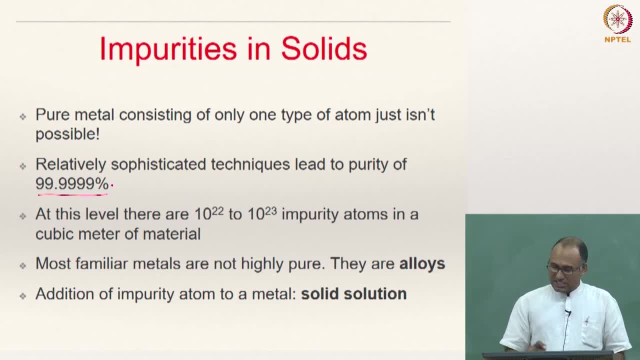 there. So at this level there are about at this 99.999% purity level you can have impurity atom of 10 power 22 to 10 power 23 in a cubic meter of material. you can have very impurity. 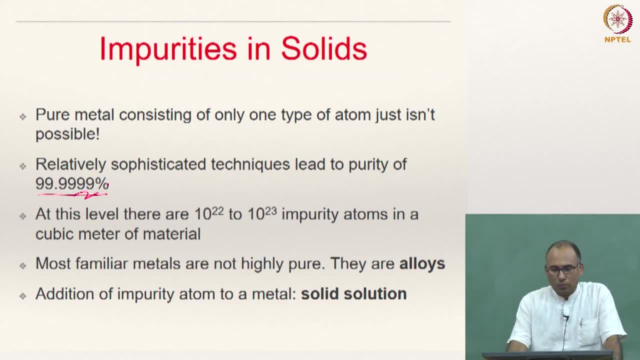 And in several engineering applications. most of the metals that we are familiar with that we are using In our engineering applications are not pure metals. they are alloys. for instance, steel is an alloy of iron and carbon, bronze and several materials you may not use them in. 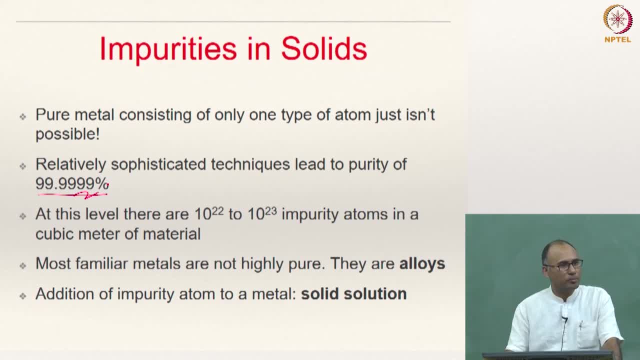 their pure form, Even when you are making your ornament. you do not make your ornament with pure gold. you add. what do you add to gold? Some of you do not know. go back and check what your goldsmith adds to gold. it is not. 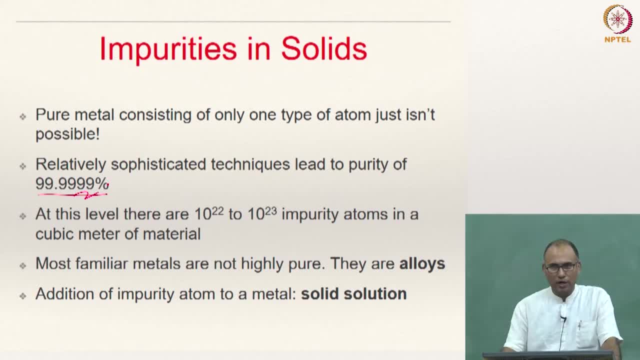 100% gold, then you make a ornament. So when you add an impurity atom to your base material, then you make a solution. right, A solution is nothing but combination of two materials. you add one material to another material. together they form solution. 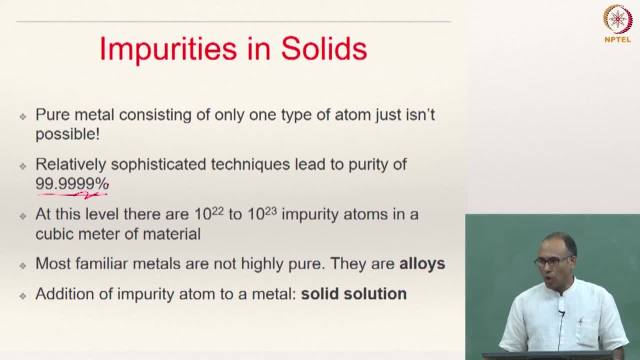 If the state of the matter is not pure, then you add impurity atom to the base material. then you make a solution. If the state of the matter is solid, then it is called solid solution. if the state is liquid, then it is called liquid solution. 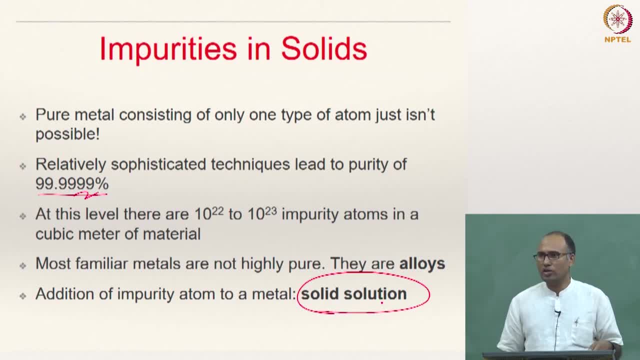 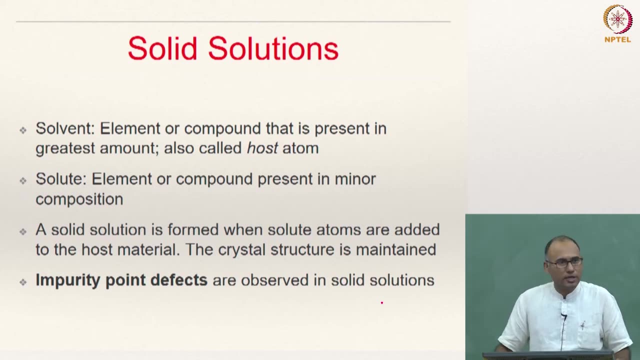 So here in this class we are going to talk about solid solution. Solid solution solution does not mean that it has to be a liquid. if the state of the matter is in solid, then you call this as solid solution. So when we are talking about solid solutions, you have a host and you have a guest. 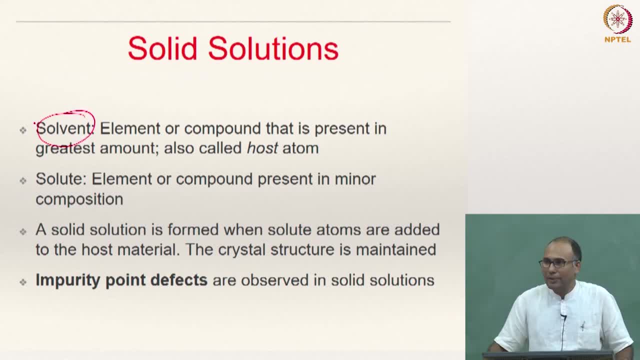 The host is called solvent. so element or compound that is present in greatest amount is called solvent and it is also called host, And the guy who is actually added to this solvent is called solute or guest right Solvent is the one which is the maximum proportion, which is there in the maximum proportion, and 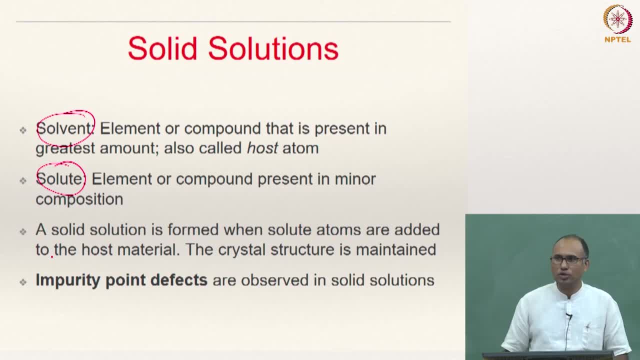 solute is the one which goes and sits there. so you add the solute to solvent. So a solid solution is formed when solute atoms are added to the host material while maintaining the structure. So you observe this impurity point defect in solid solutions. 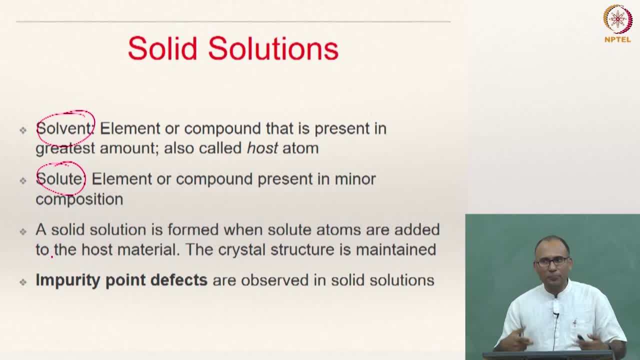 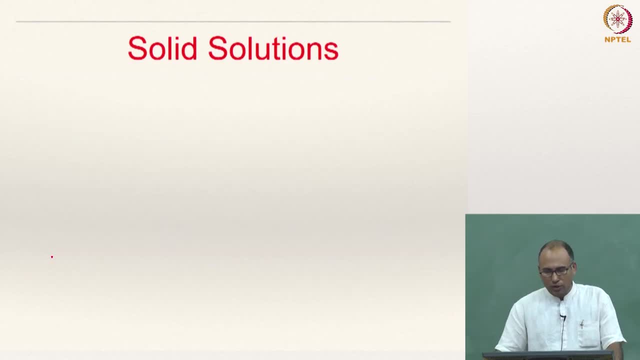 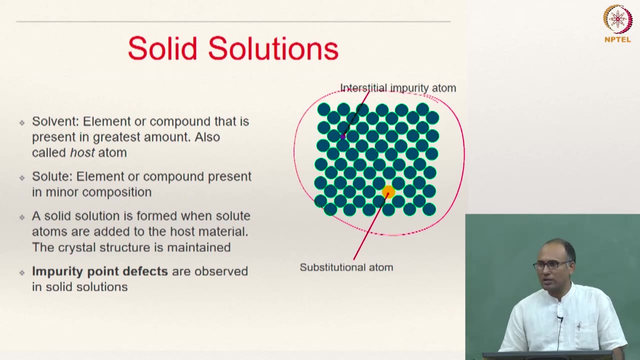 A solid solution is actually something in which we intentionally add point defects, right? So if you look at so, let us say this is a crystal lattice, The green ones are your crystal lattice, And now you can see two different kinds of point defects. 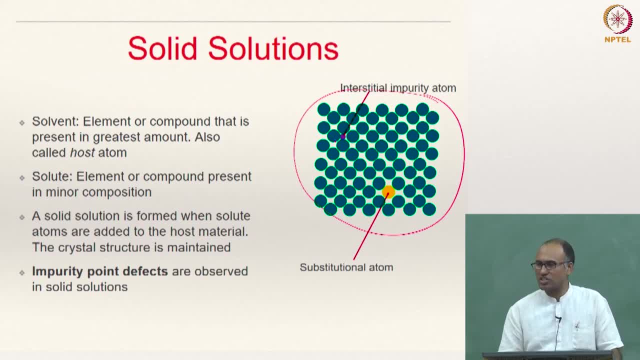 One point defect is a point defect is actually going and sitting in the interstitial location, Then it is called interstitial impurity atom And if it is going and sitting in the substitutional position, it is substitutional impurity atom. that we have discussed already previously. 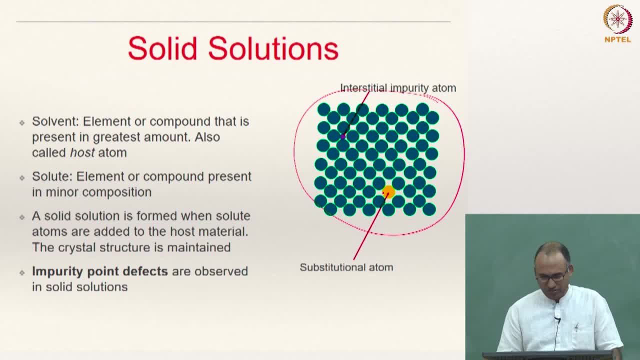 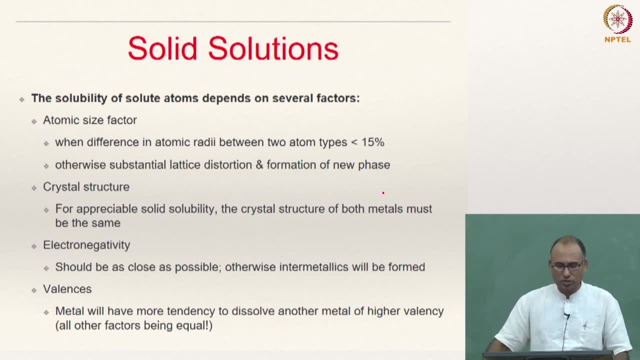 And we are talking about different kinds of point defects, right? So what are different kinds of? how do you actually go about forming this solid solution? So the solubility of solute atoms, So the solute atoms actually need to be, need to go and sit in solvent atmosphere. 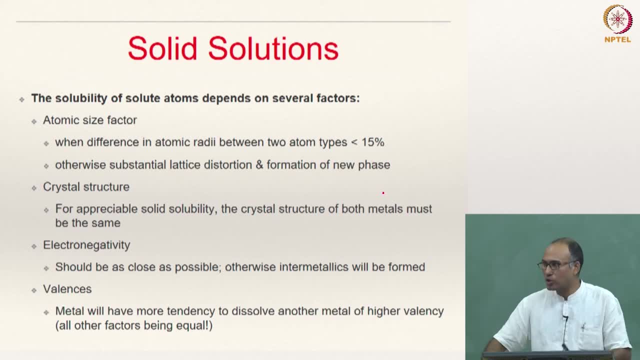 That means there should be some amount of solubility for this solute atom in solvent atmosphere, right? Otherwise it cannot go and sit there. So this solubility depends on several types. okay, First of all, atom size factor. 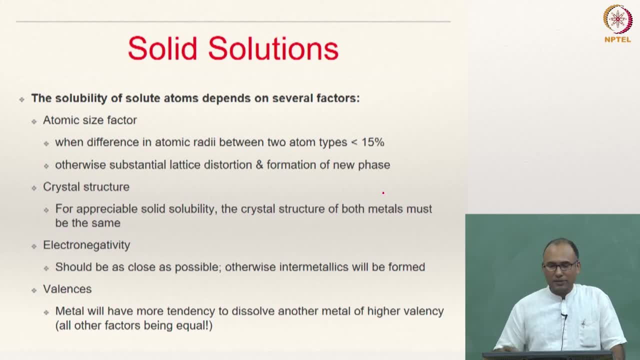 If there is a solubility, What happens? What is the difference between the atomic sizes If you are forming an interstitial solid solution, meaning all your impurity atoms are actually going and sitting in the interstitial locations of your solvent cloud? 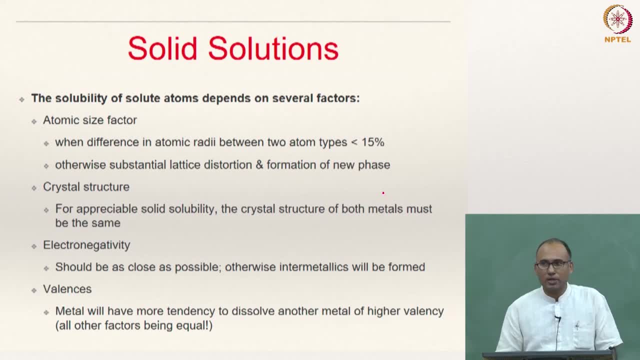 That such a solid solution is called interstitial solid solution. If your solute atoms are going and sitting in the substitutional positions, they are actually going to substitute for your solvent atoms. Then such a solid solution is called substitutional solid solution. okay, 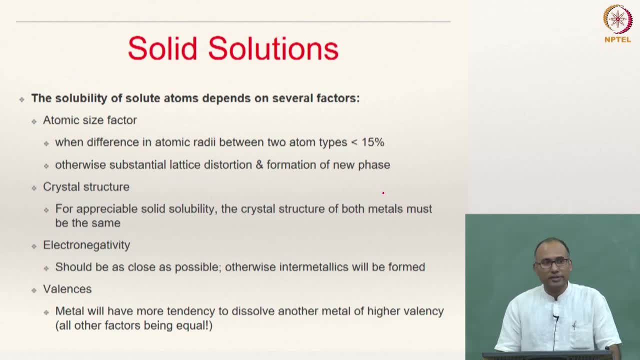 So when do you form a substitutional solid solution or interstitial solid solution? That actually depends on several factors. One of the important factors is atomic size factor, When the difference between difference in the atomic radii sizes is less than 15% only. 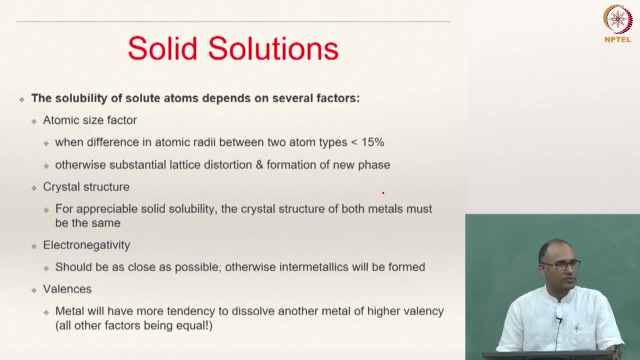 then you will be able to form substitutional solid solution. Otherwise you cannot form a substitutional solid solution. Okay, Otherwise you will form interstitial solid solution or you will create lattice discharge. And for a good solid solubility, the solvent atom and solute atom should be having same. 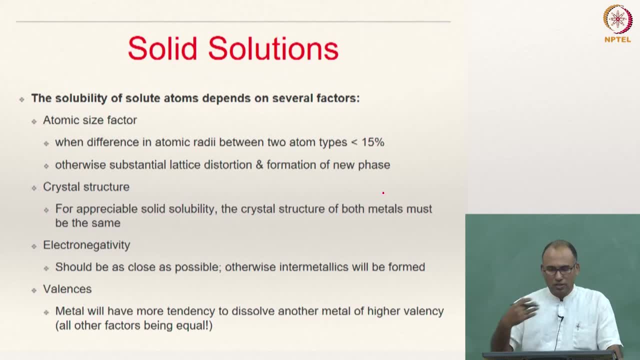 crystal structure. If they have similar crystal structure, then the solubility is better And their electronegativity values should be as close as possible. They should not have large difference in their electronegativity. Okay, And the valence is also another important thing. 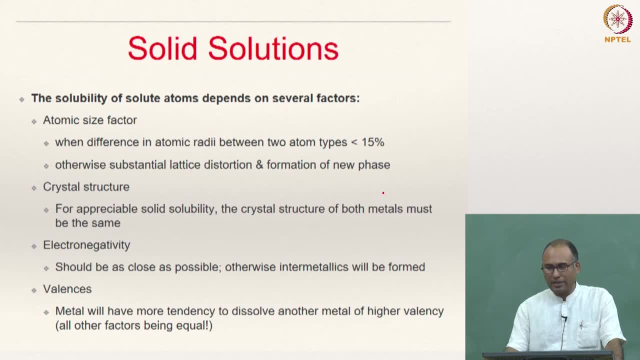 So metals will have more tendency to dissolve another metal of higher valence right, While, all other factors being equal, it actually tries to. so this is not the primary thing. When all other things are satisfied, then it will look for a metal to dissolve a metal. 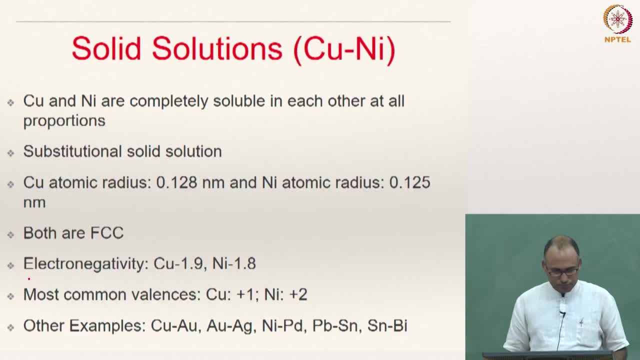 which has higher valence than itself. Okay, So one very important thing, So one very good example for substitutional solid solution is copper- nickel system. Copper and nickel are completely soluble in each other at all proportions. If you take 90% copper, 10% nickel and vice versa, so they are completely soluble in each 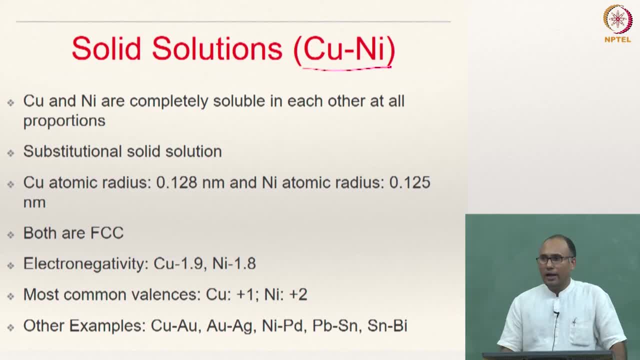 other Right And it forms a substitutional solid solution. You can see why The copper atom radius is 0.128.. Nickel atom radius is 0.128.. Okay, The copper atom radius is 0.128.. They are very close to each other. 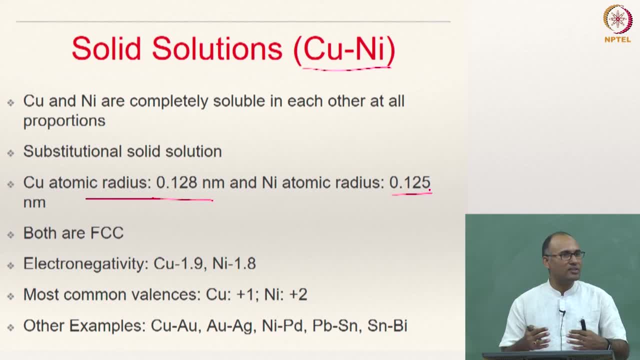 That is why their solubility is: first of all, they are close to each other and hence they will only form substitutional solid solution. right, because the interstitial sides are going to be smaller for them, because the atom sizes are almost same. 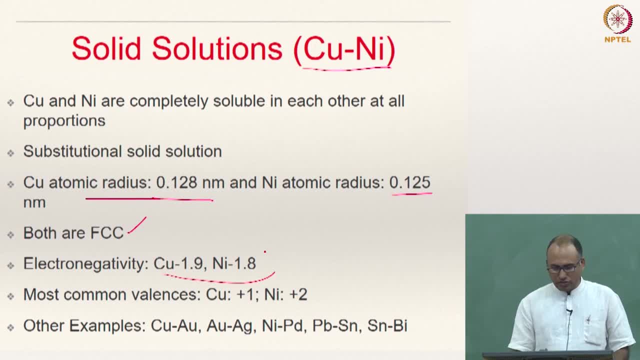 Both are FCC and their electronegativity values are also very close: 1.9 and 1.8.. And hence they form a very good substitutional solid solution with 0.128.. Okay Okay, They form a very good solution with almost complete solubility: 100% solubility in each. 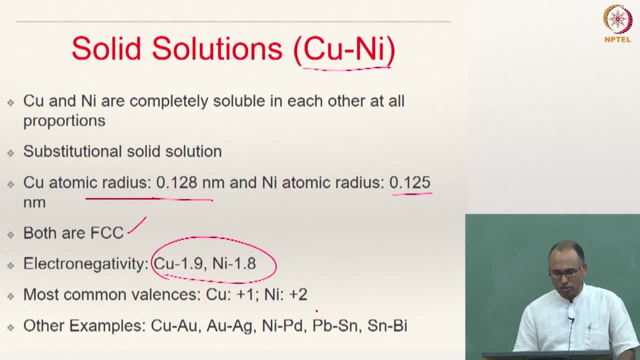 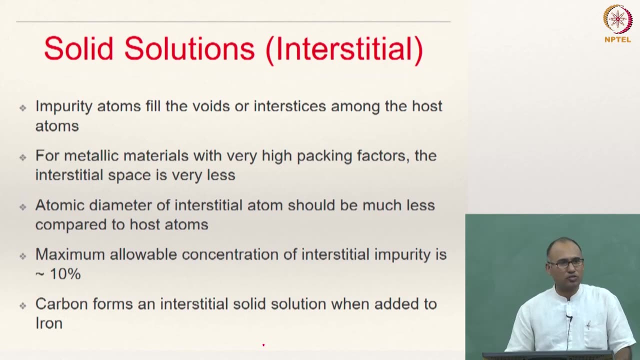 other Other examples for substitutional solid solutions are copper, gold, gold, silver, nickel, palladium, lead tin, tin, bismuth and so on. Right, And what are the examples for interstitial solid solution? So when do you have interstitial solid solution? 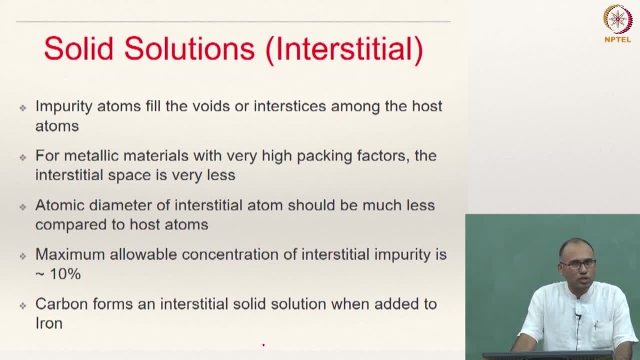 When the guest atom or the solute atom size is 0.128.. Okay, When the solute atom size is smaller, much smaller than the solvent cloud, and then it actually can go and sit in the interstitial position. So impurity atom still, the voids are interstitial among the solute solvent cloud or host material. 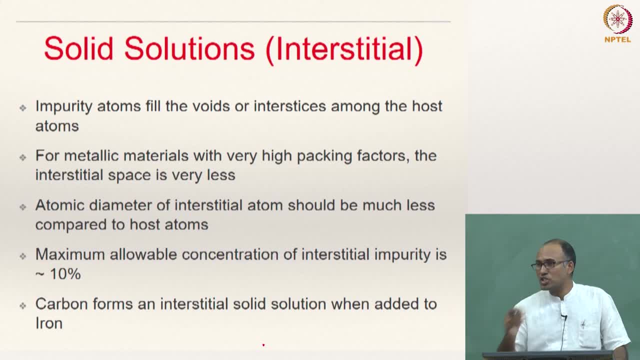 Okay So but the when you have an interstitial solid solution, you cannot actually have complete solubility. So here you have. the maximum allowable concentration of an interstitial impurity in general is only above about 10%. You cannot actually dissolve a material which will form an interstitial solid solution more. 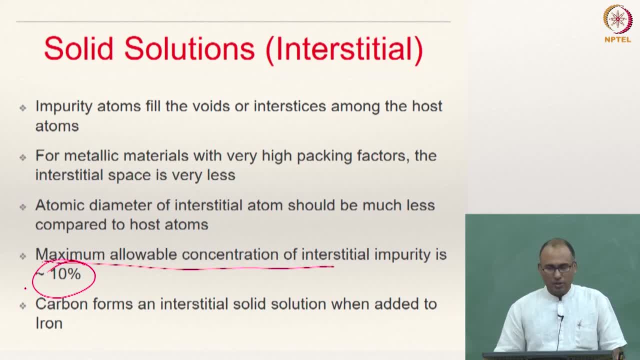 than 10%. Okay. So, for instance, carbon forms an interstitial solid solution with iron, So steel is an interstitial solid solution of iron and carbon. Okay, And the maximum allowable, so maximum solubility of carbon in iron is 2%, not more than that. 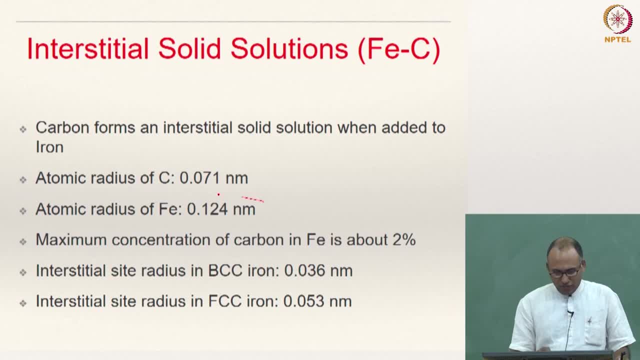 Right. So you see that atomic radius of iron is 0.124 and this guy is much smaller, 0.071, and that is the reason why it actually can nicely go and sit in the interstitial location. And the maximum carbon concentration of carbon in iron is about 2%. 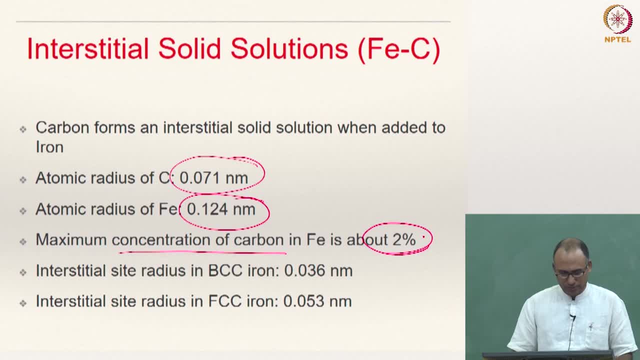 2 point, something So about 2%, And if you carefully look at it, the interstitial suppose. iron can occur in two forms. Right You have alpha iron and gamma iron. Right, Alpha iron is BCC, while gamma iron is FCC. 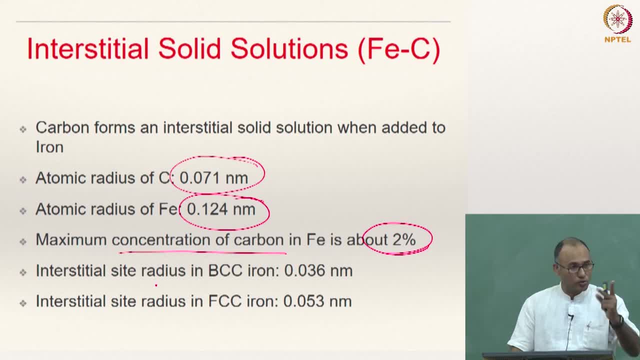 Right, Okay, FCC. You will have two different structures. It changes its space depending on the temperature and composition. So if you look in BCC material iron lattice, you will see that the interstitial site radius is 0.036 nanometers by knowing the radius of iron. and if it is FCC then you have 0.053. 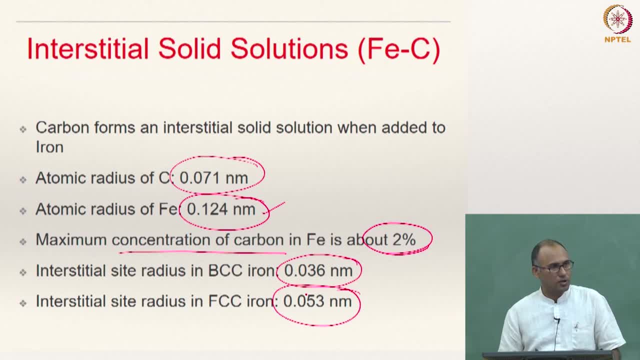 nanometers, All right. So please note that the carbon is actually going and sitting in the interstitial site, But the size of carbon atom is actually larger than any of these, Right? So when actually carbon goes and sits, it sort of disturbs the crystal lattice locally. 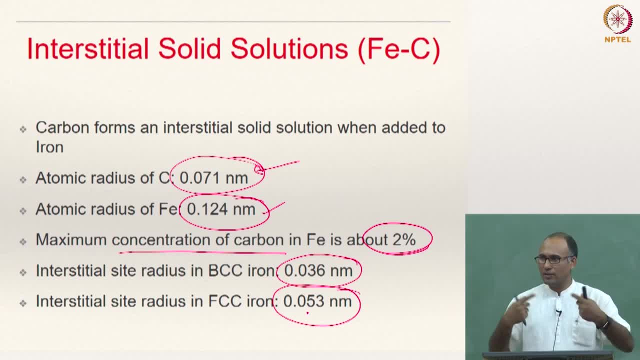 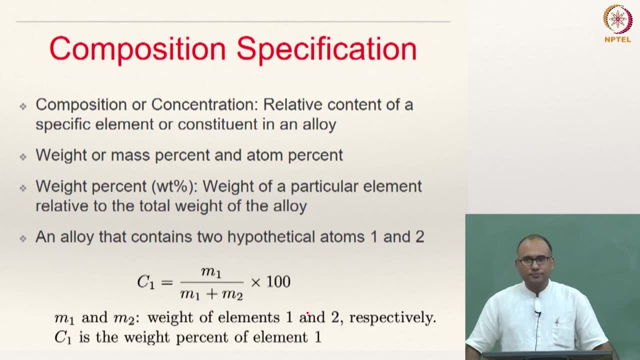 It will create local distortion and hence the energy of the crystal might shift because of the local distortion. All right, Let us, we will discuss about it when we are talking about phase diagram. Okay, At this point of time I am not discussing that, but we will discuss when we are talking. 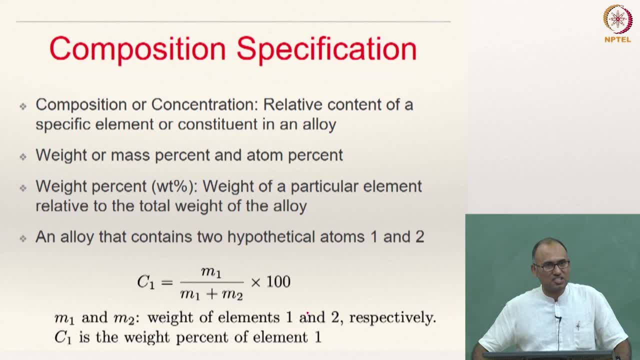 about phase diagram. The question is: why does iron change its crystal structure when you go from one temperature to another temperature or composition? Okay, That is what I said Iron has. it is called alpha iron at low temperatures and gamma iron has little high temperatures. 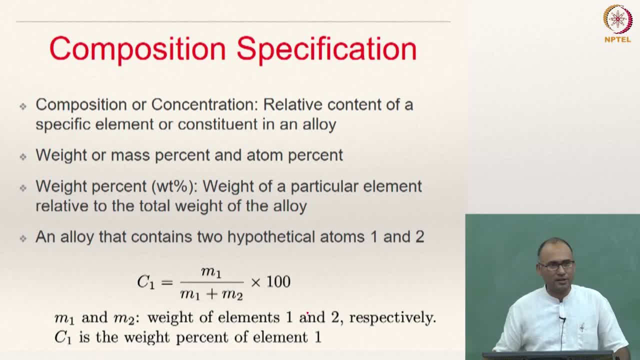 and again, much higher temperatures. again it becomes delta iron BCC again. So why does it change crystal structure? we will discuss, Maybe towards the second end of this course. Yeah, Okay, Now you have a solid solution. and now how do we specify the composition or concentration? 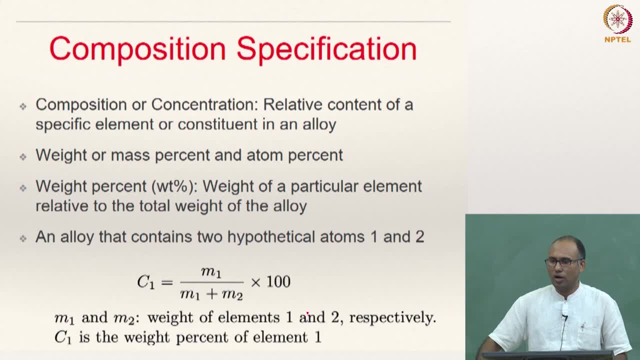 So the relative content of a specific element or a constituent in an alloy is called the composition. Okay, So you can describe this composition as weight percentage or atom percentage. What do you mean by weight percentage? how? what is the meaning of weight percentage? 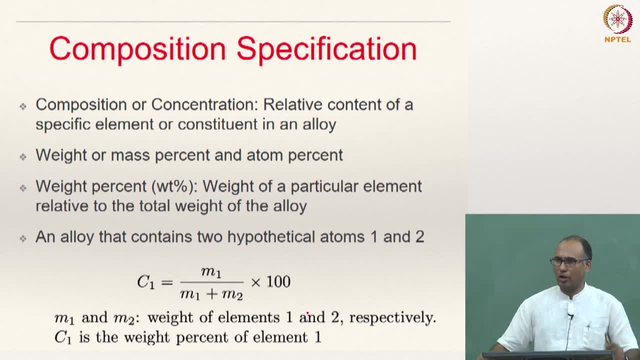 The weight of a particular element relative to the total weight of the alloy. What is the atom percentage? Instead of weight, you only talk about the number of atoms. Right, The fraction of number of atoms. then it is called atom percentage. we will see the definition. 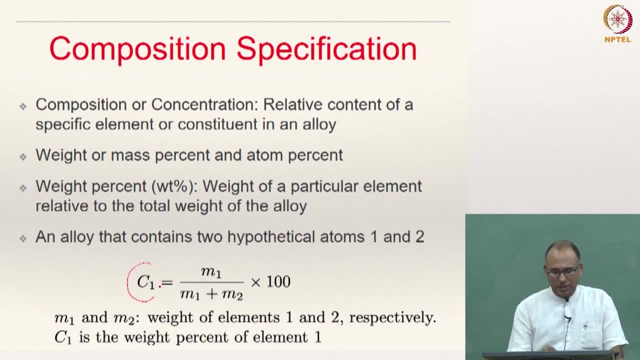 in a moment. So the composition of an element 1 in an. suppose if you have a binary alloy. What do you mean by binary alloy? You have only two elements, one solid and one solvent. Okay, If you have a binary alloy made of element atoms 1 and 2, the composition: weight, percentage. 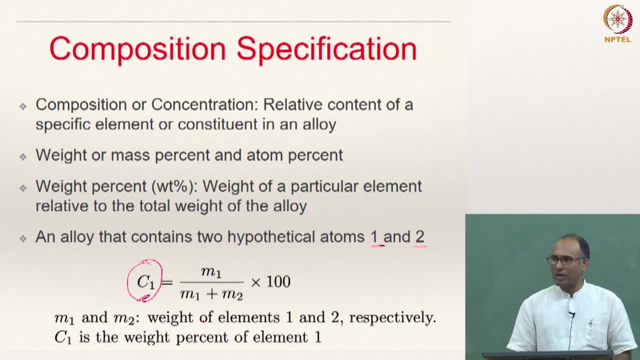 in weight percentage can be defined as m1 by m1 over m1 over m2.. Okay, Okay, 1 plus m2 times 100.. So that is your. that is the regular definition that you have studied in your high school. 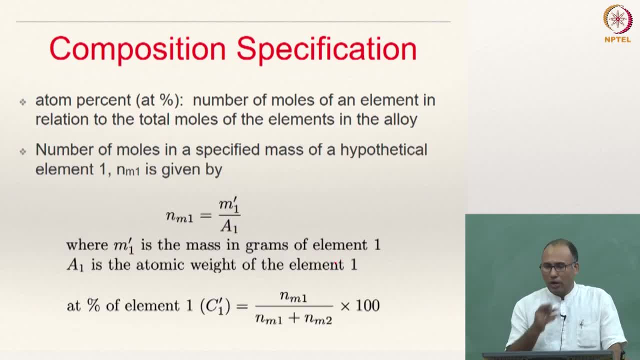 before coming here. Right, If you want to define atom percentage number of moles of an element in relation to the total moles of the element in elements in the alloy, So number of moles can be defined as mass of that particular species divided by the. 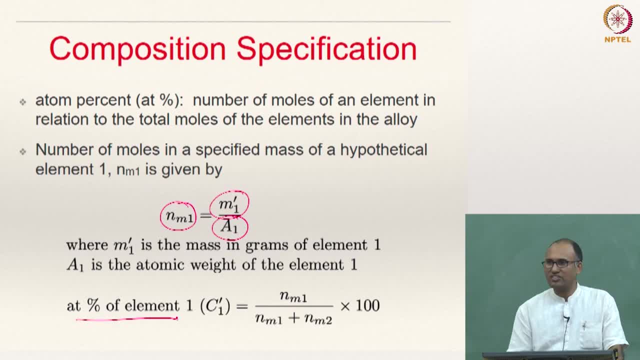 atomic weight of that particular species, And hence atom percentage can be defined as nm1, that is, number of moles of atom type 1 divided by the total number of moles, that is, nm1 plus nm2.. Right, So you can define, so you can actually express the composition, either in weight percentage. 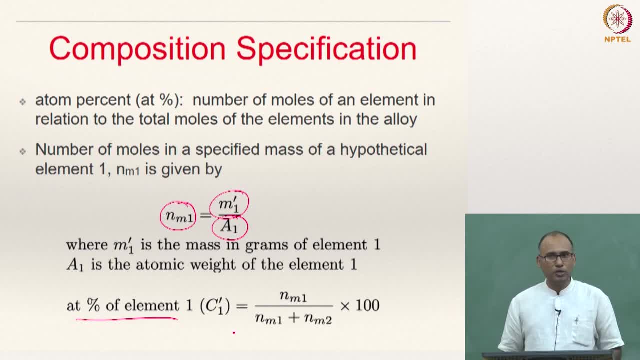 or in atom percentage. So when you look at these composition diagrams you will either have weight percentage or atom percentage. Sometimes you will have both of them. So if you draw the diagram On the bottom x axis, you will have the weight percentage or the atom percentage. 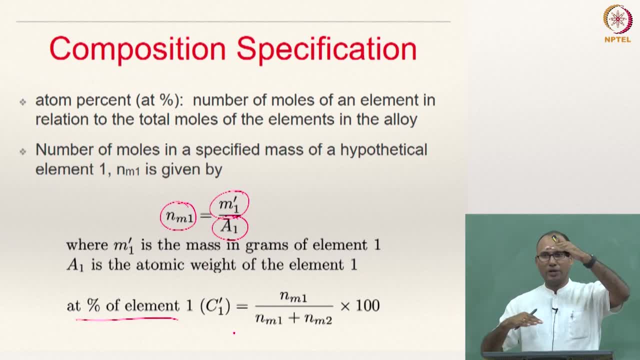 Sometimes you will have both of them. So if you draw the diagram, On the bottom x axis you will have weight percentage and the top x axis you will have atom percentage. So in the same diagram you can see you can actually make this. you can read the diagram. 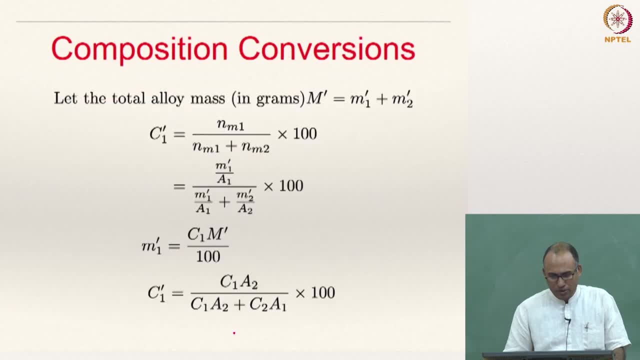 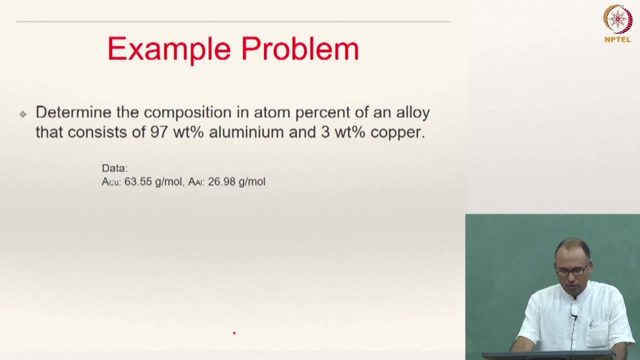 either in terms of weight percentage or atom percentage. Okay, So I am not going to discuss these derivations, but you should be able to convert from one to the other by knowing the atomic weights of this material. Okay, So to here. I am not going through that. we will do through tutorials, but the slides 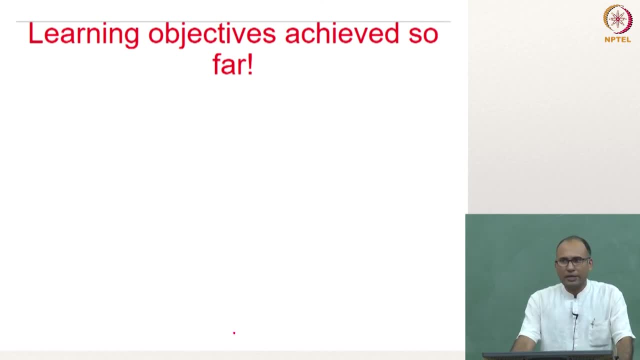 are there So you can actually go through the slides. Okay, So that is about point defects. So what did we learn so far? Now can we list different types of defects in a solid Yes or no Louder? 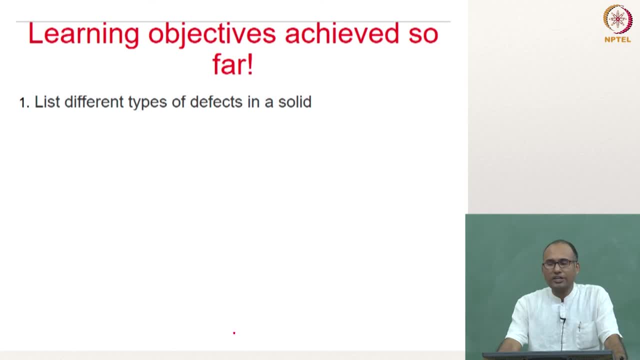 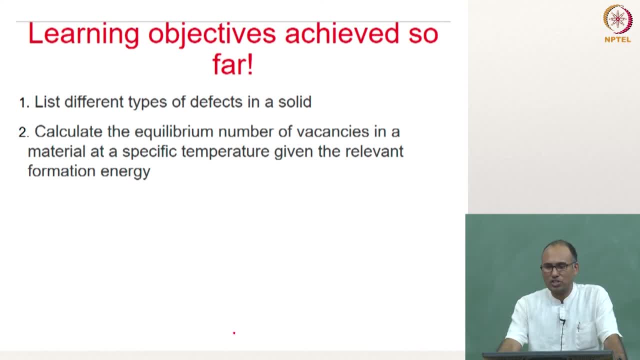 Yes or no? Yes or no, Yes or no. Can we list the concentration of vacancies in a material at a specific temperature, given the relevant formation, energy We can calculate. Can we derive the expression for equilibrium concentration of vacancies? Can we list different types of solid solutions? 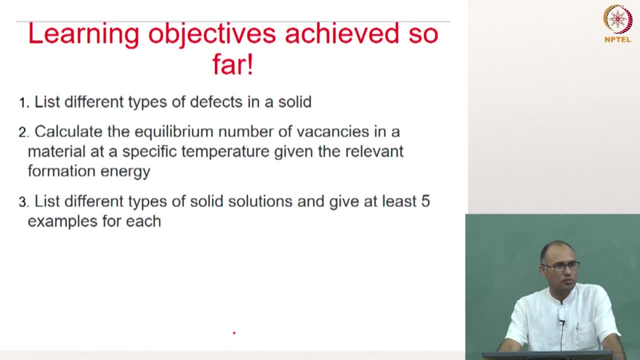 Today we have looked at substitutional solid solutions and interstitial solid solutions, and can we give at least 5 different examples for each? We have already given 5 examples for substitutions. Okay, substitutional solid solution: copper, gold, gold, silver, right. 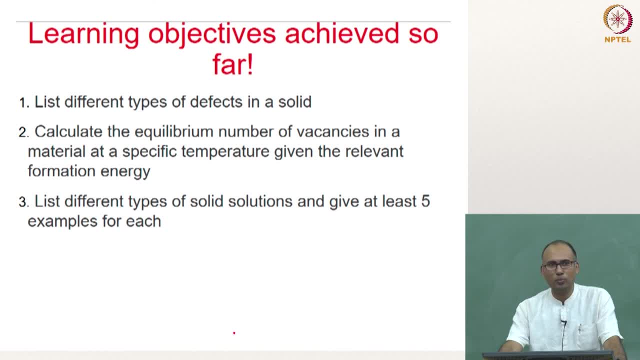 And I have given you one example for interstitial solid solution, but you should be able to go back and find out what are the other materials which forms interstitial solid solution. other alloys that you are familiar with are actually interstitial solid solution. And you, what are the conditions for the formation of either a substitutional solid solution? 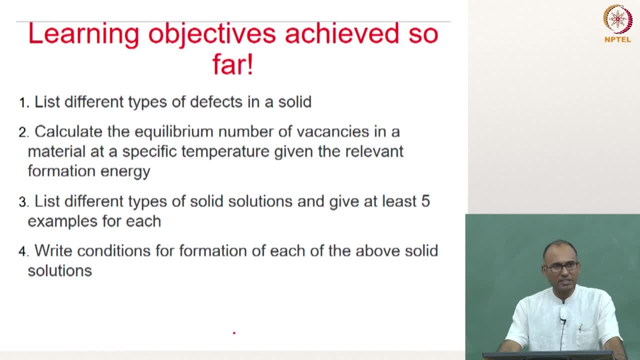 or an interstitial solid solution. So we have looked at the atomic size factor, electronegativity- what else? valency state and crystal strength. So these are the things. So based on that, you can actually decide whether a material is a particular system. 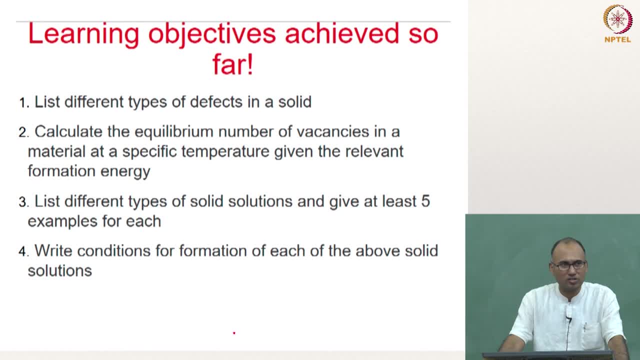 is more probable to form a substitutional solid solution or an interstitial solid solution, And we should be able to calculate weight and atomic percentage of elements of an alloy. If you know the volume fraction, then you should be able to calculate weight and atom. 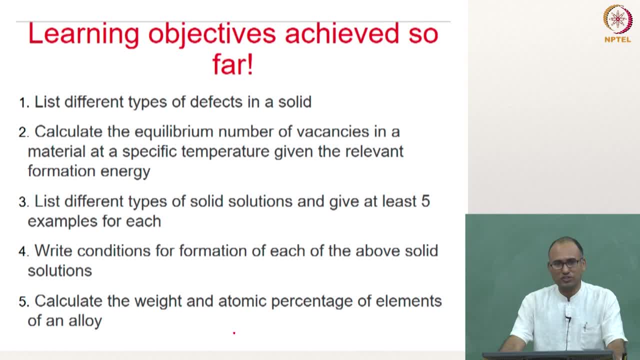 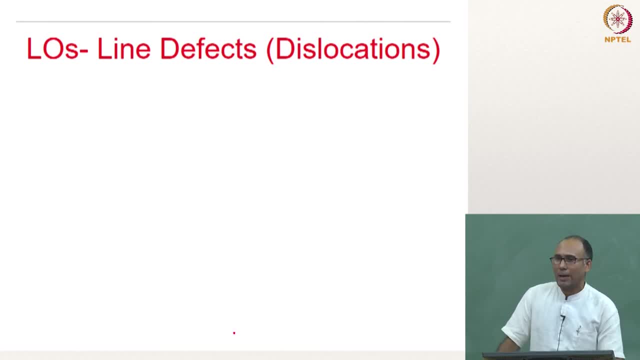 percentage. So that is what we have looked at so far. So we have looked at the zero dimensional defects. Now we need to focus our attention on line defects or one dimensional defects. So these line defects are also called dislocations. 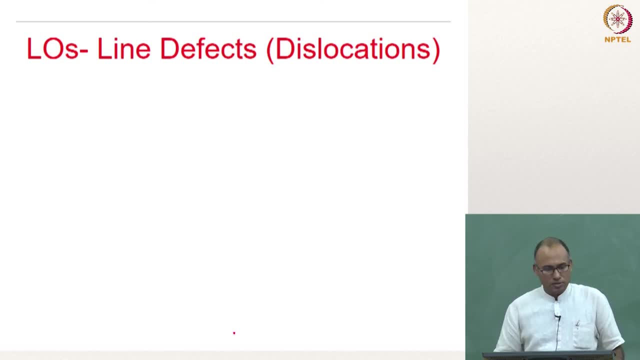 So what are the concepts that we are going to learn in this module? First of all, you should be able to draw a schematic of the line defects. So what are the lines? What are the lines? What are the lines? As an example, there is a line that is a. 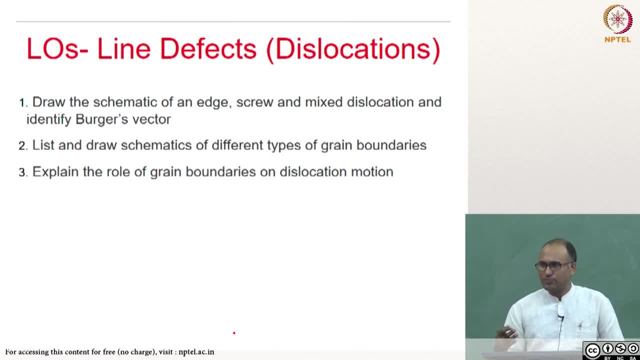 Reading program we had 10 to 12 lines like that. If i submit this as 16 to 17 lines, then you can identify this line as this: This line is not a Halven founder line, So this average line vector has finished breaking down to 12.. 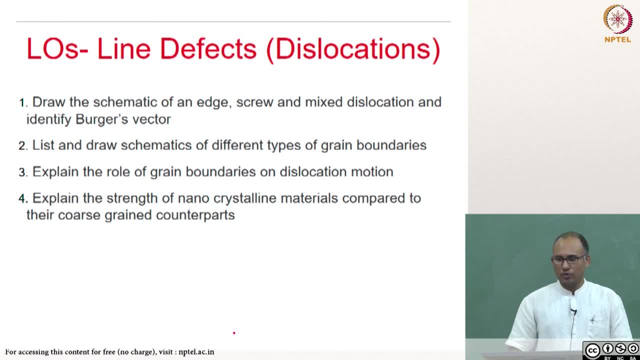 So now you can calculate the 0 and 25, three sides of the 270 nanometer net. Ok, That is it, with the knowledge gained until here, to explain the strength of nanocrystalline materials compared to their coarse-grained counterpart. 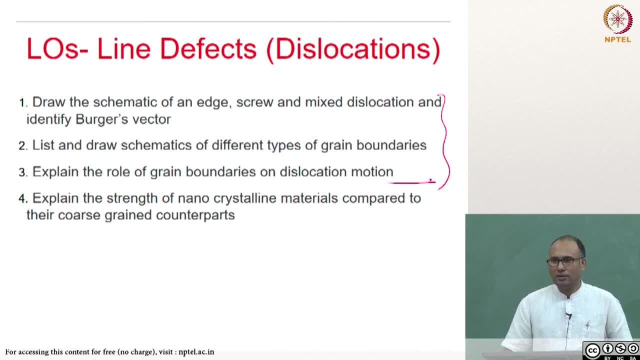 Why a nanocrystalline material is much stronger than the coarse-grained counterpart. okay, Nanocrystalline copper is stronger than normal copper- polycrystalline copper, normal copper. Why is that? We should be able to explain that. 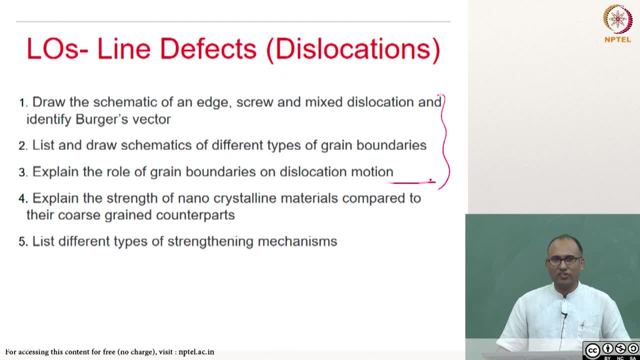 And what are the different types of strengthening mechanisms? What do we mean by strengthening? We will discuss. So we should be able to list different types of strengthening mechanisms and plot the schematic variation of these mechanical properties as a function of weight. percentage of alloying. 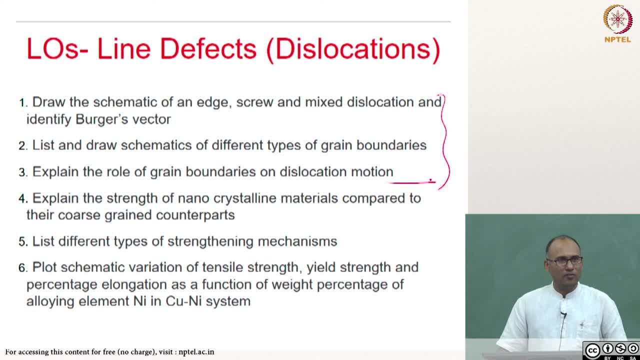 elements. We have just now seen that you have a substitutional solid solution and an interstitial solid solution and, depending on the composition, how your mechanical properties change. And finally, we should be able to derive the expression for critically resolved shear stress to talk about plastic deformation in a material. all right, 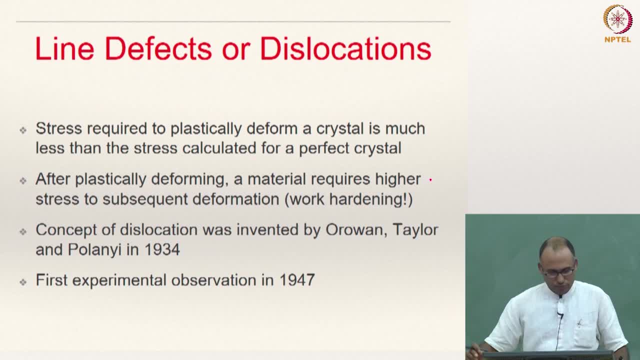 Okay, I will just introduce you to the concept of the line defects and then we will stop. okay, But we can again start at the same point tomorrow. We have- we know that- the stress required, as we have discussed in today's class, as 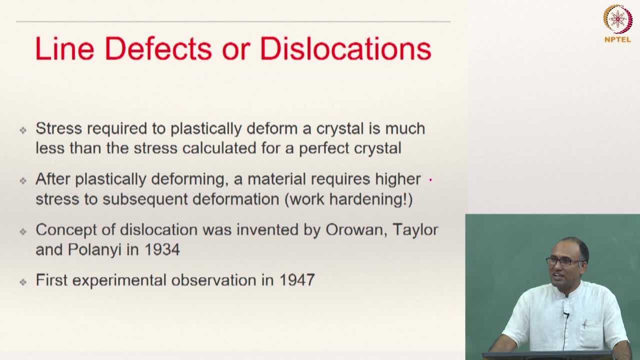 well as in today's class. the stress required to plastically deform a crystal is much less than the stress calculated for. a theoretical shear strength we have calculated sounds out to be much larger than the real shear strength of the material, So the shear strength was less than the shear strength of the material. 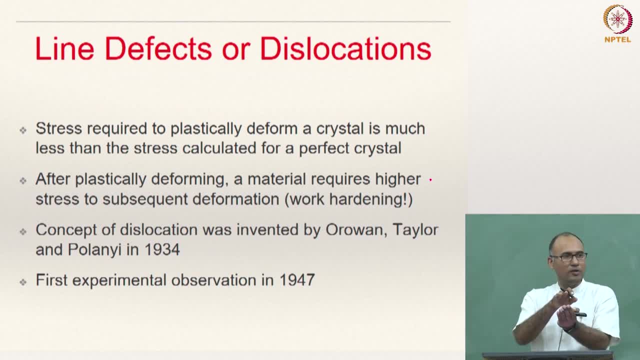 Okay, So the shear strength- the reason why we call that represents the plastic deformation- is basically because your, this atom, one atom which is in contact with a set of atoms, is actually going away from these atoms. so that means this: the neighbors of these atoms. 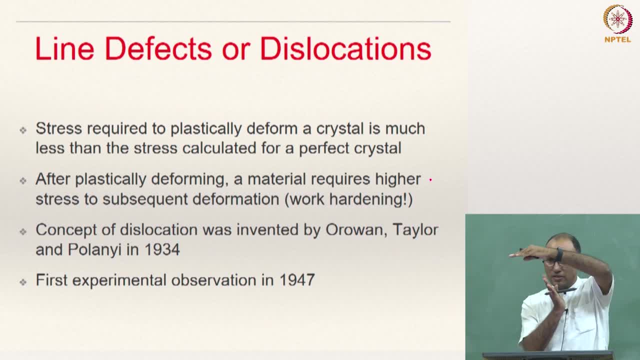 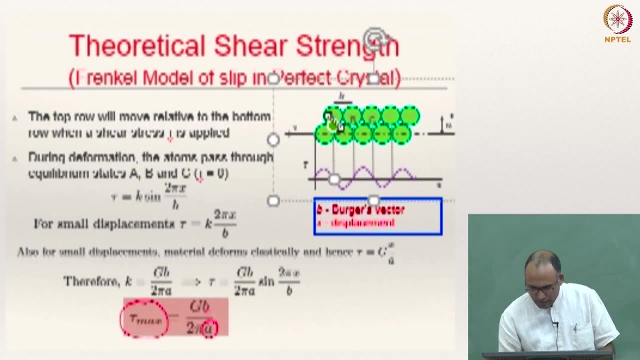 are changing, right When you are before applying the shear stress. if you remember, if you remember this picture, for instance, this atom A here, right When it moves, Okay, When it moves, when you are applying the shear stress, this atom A is actually in contact. 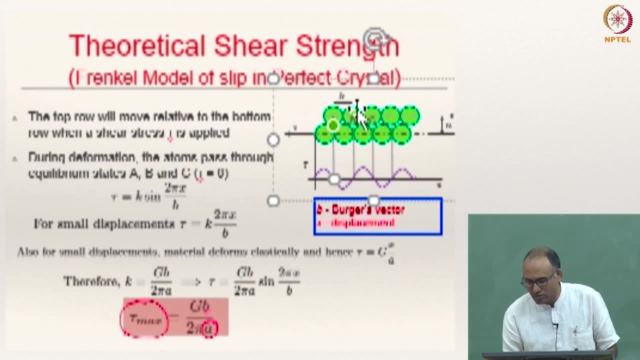 with this first atom here. but when you are applying shear stress this atom A actually moves to the position B right And then its neighbor is changed. that means it there is a breakage of bond And that means once you remove the shear stress there, it will never be able to come back. 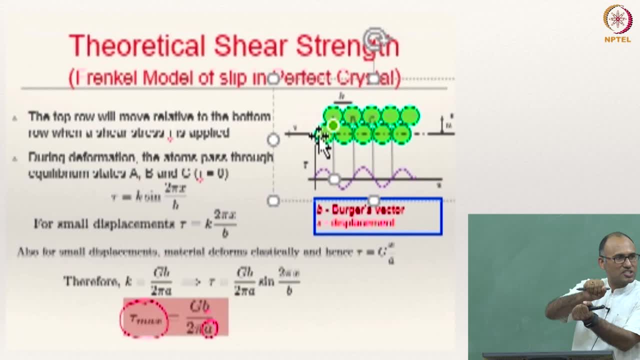 to its original configuration, And that is what we call plastic deformation. Plastic deformation is non-reversible- Okay- Whereas elastic deformation is reversible. When you are applying load- external load- to a material first, what you do is you actually stretch the bonds before you break them. 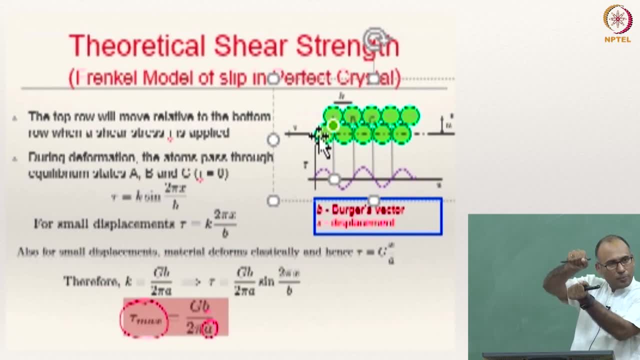 Before breaking them. if you remove the load, then the bond- elastic bond- is retained and hence it will come back to its original configuration. That is the reason why, under elastic regime, within the elastic regime, when you remove the load, the material comes back to its original configuration. 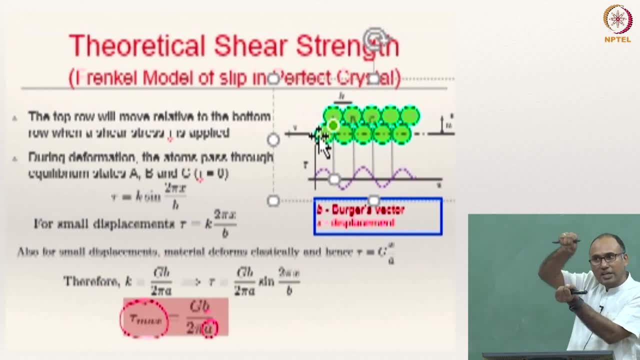 But then you are going on. Okay, When you are going past that area, then what you are actually doing is you are actually breaking the bond here. Once you break the bond, energy is dissipated and then after that, if you remove the load,